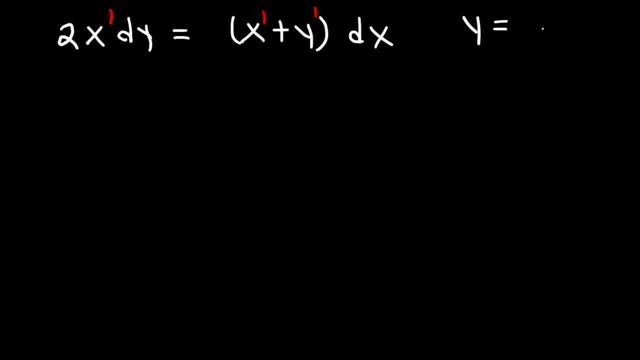 Now, whenever you have this situation, what you want to do is replace y with v times x And at the same time, you need to differentiate this function using the product rule. The derivative of y is dy And to differentiate vx. you need to differentiate the first part. 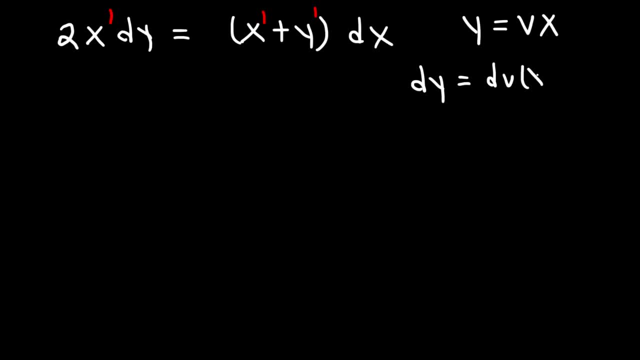 The derivative of v is dv, and then times x, And then now we need to differentiate the second part, keeping the first part the same. So the derivative of x is dx. So we can say that dy is x dv plus v dx. 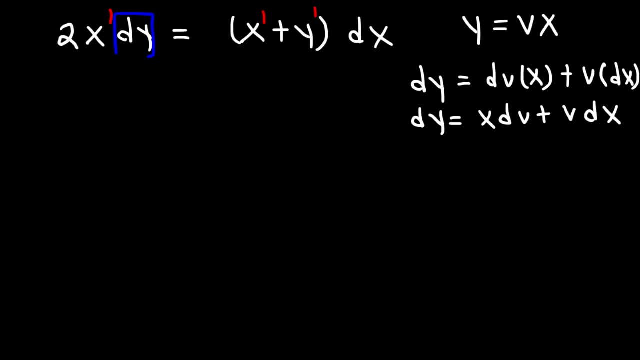 So let's replace dy with this expression And at the same time let's replace y with v times x. So this is going to be 2x times x dv plus v dx, And that's equal to x plus vx times dx. 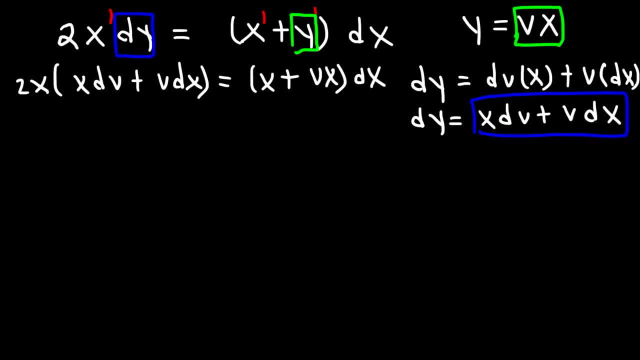 So now what we want to do is we need to do is simplify. for now, I'm gonna leave the left side the same. there's no need to change it at this instant. now, the right side: I can factor out an X, so I'm gonna have 1 plus V times DX left over, and so I could divide. 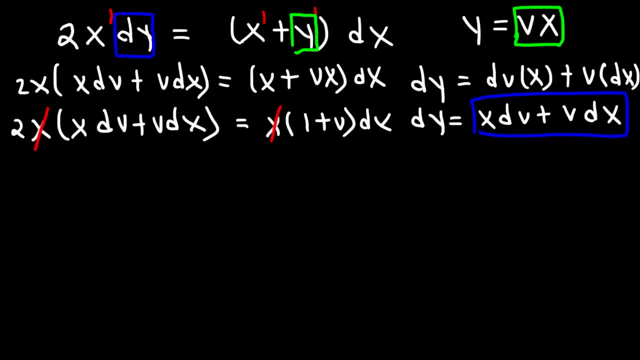 both sides by X or just cancel the X variable and I'm gonna distribute this 2 to everything inside here, so it's going to be 2x DV plus 2 V DX. on the right side, I'm going to distribute DX to 1 plus V, so it's going to be 1 times DX. 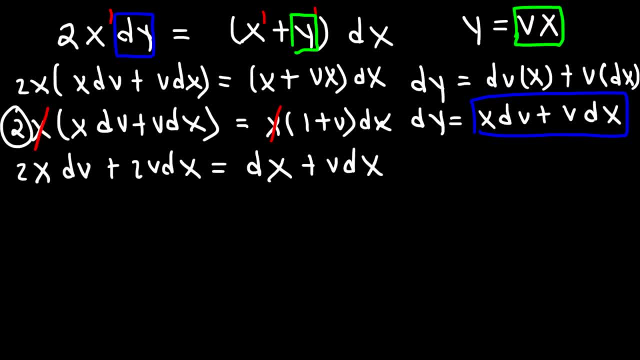 which is DX, and then plus V DX. so notice that these two terms are similar. we have a 1 in front of this term, so I'm going to subtract both sides by X, 1 times V DX, and so this will cancel, and now I have 2x DV. 2 minus 1 is 1, so 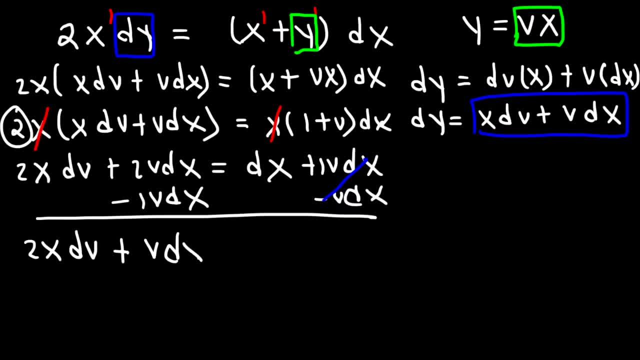 plus 1 V DX, or simply VX, and that's equal to DX. now I'm going to take this term, move it to the other side, so we have 2x DV and that's equal to DX minus VX, V- DX. now, on the right side, I'm going to factor out DX, so it's gonna be 1 minus. 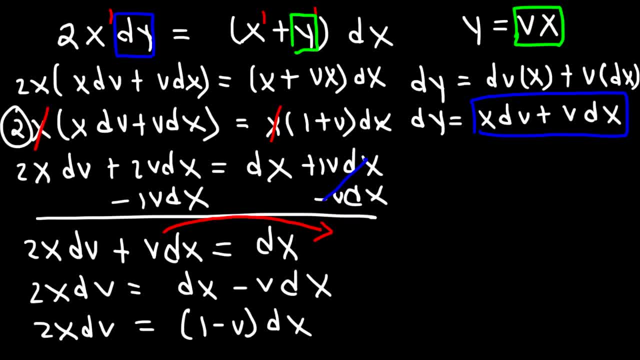 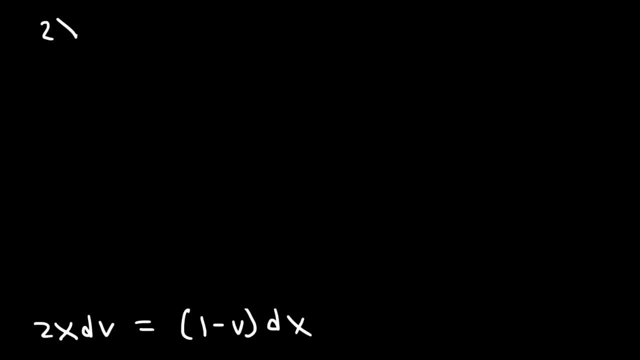 V times DX. so what I'm going to do at this point? let me just rewrite this equation at the top: I need to separate the variables you. So how can I do that? How can I separate x from v? At this point, you need to divide both sides by 2x and also simultaneously by 1 minus v. 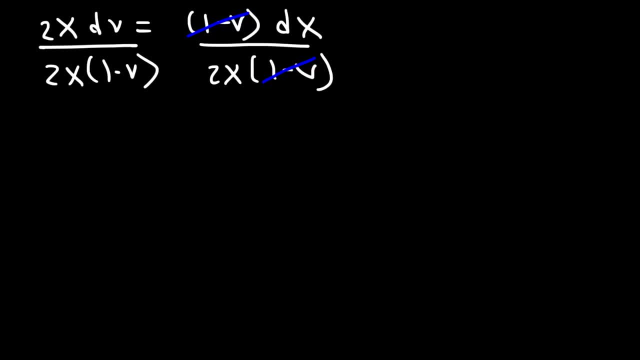 So on the right side the 1 minus v term will cancel and on the left side 2x will cancel. So on the left I have 1 over 1 minus v times dv and on the right 1 over 2x dx. 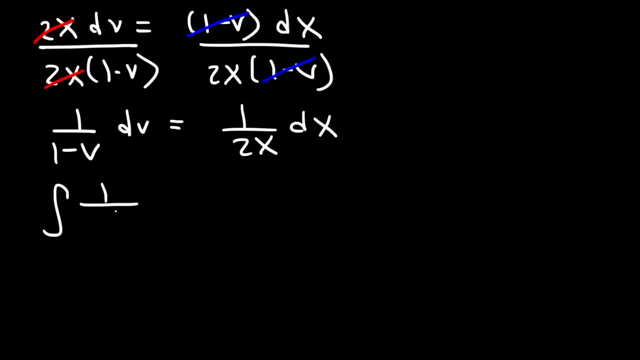 So now I can integrate both sides. So on the left I have the integral of 1 minus v dv. On the right I'm going to take out the 1 half, put it in front of the integral symbol. So I have 1, half the integral of 1 over x dx. 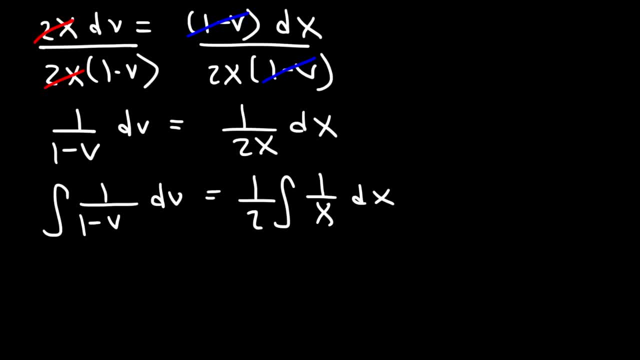 So what is the antiderivative of 1 over 1 minus v? Okay, And what is the antiderivative of 1 over x? The antiderivative of 1 over x is ln x, And the antiderivative of 1 over 1 minus v is ln 1 minus v. 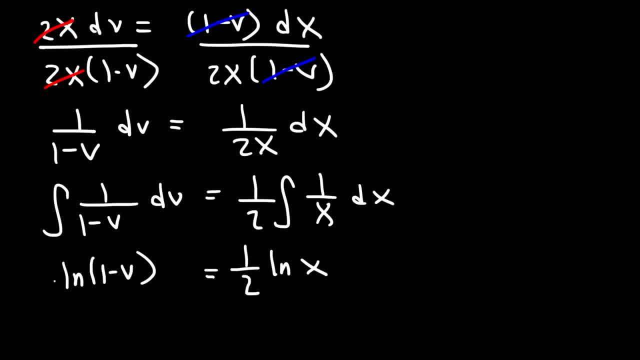 But if you take the derivative of 1 minus v, that will give you negative 1.. So we need to put the negative in front And then, on the right side, I'm going to add the constant c. So this is what we now have. 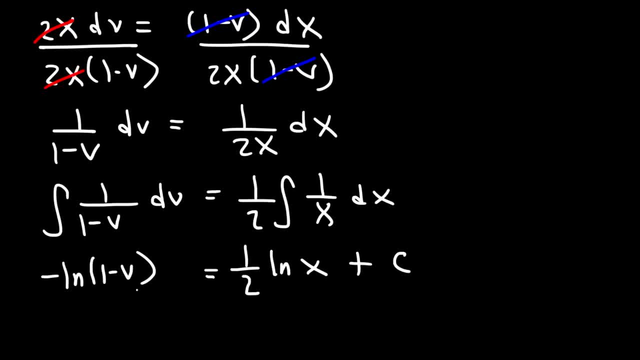 Now we need to clean up. We need to clean up our solution. So what do you think we need to do? This negative sign- you can view it as the negative 1 in front of the natural log expression And the property of logs- allows us to take the coefficient and move it to the exponent. 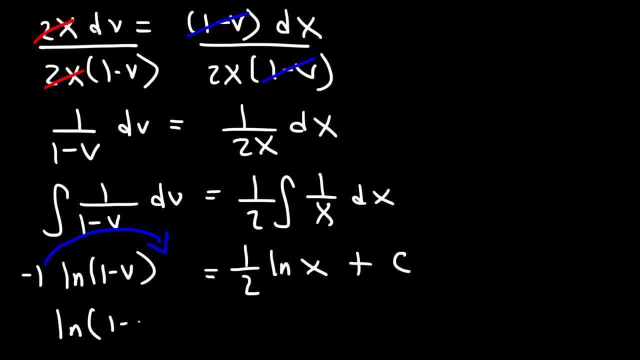 position. So this is ln 1 minus v raised to the minus 1.. And I'm going to do the same thing with the 1 half constant. So this is going to be ln 1 minus v raised to the minus 1.. 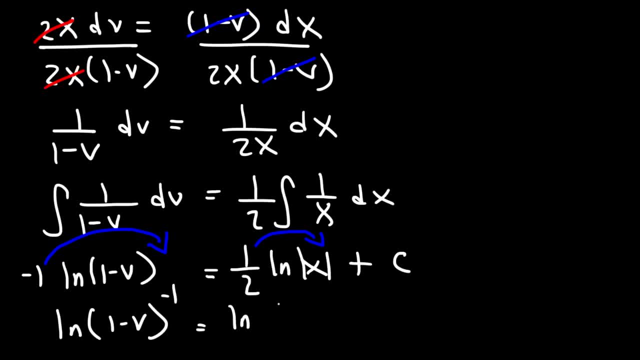 Right now it's an absolute value of x, And then it's going to be square root x or x to the 1 half, which I'll leave it as x to the 1 half for now. Now c, I'm going to put a natural log in front of it. 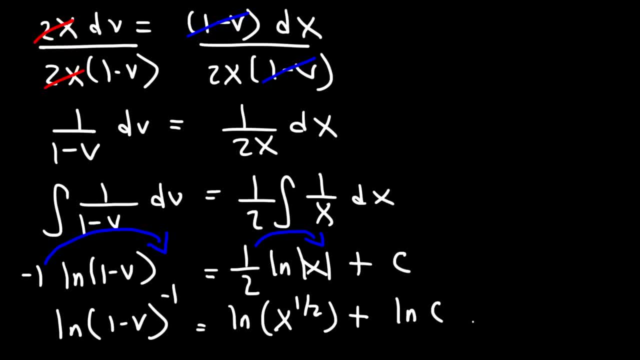 ln c and c. they're both constants, So I can just make it natural log of c. It's still a constant. If I differentiate c or ln c, the result will still be the same. It will give me 0.. So that's it. 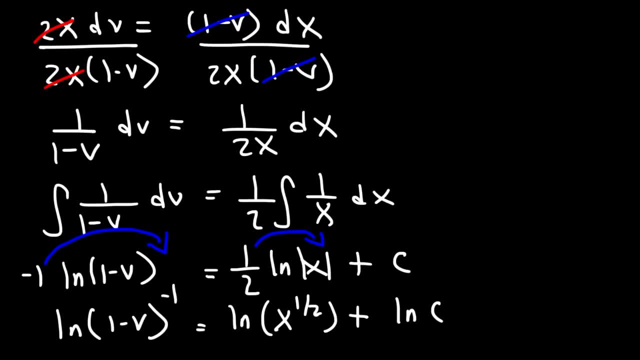 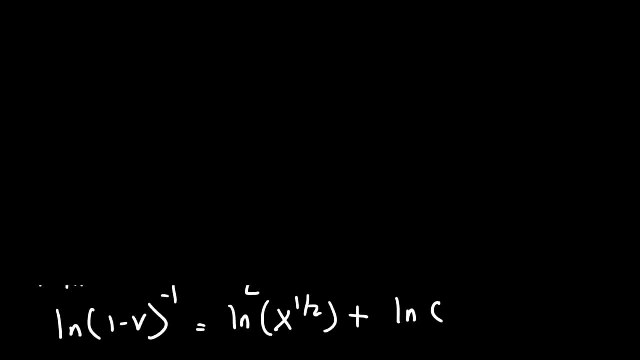 So this doesn't change the answer. Now, 1 minus v raised to the minus 1 is the same as 1 over 1 minus v, And on the right side we have the natural log of the square root of x plus ln c. 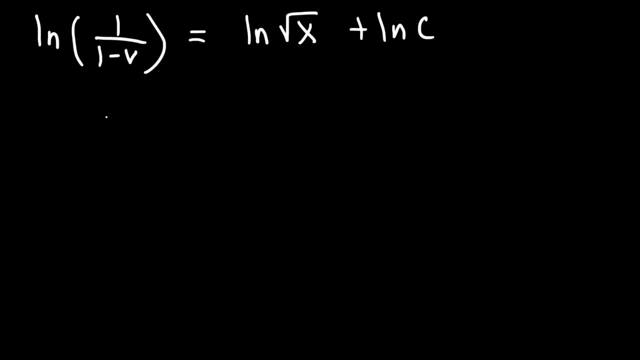 Now we need to condense those two logs into a single log. For instance, ln a plus ln b can be written as ln a times b, So ln square root x plus ln c. we can write that as ln c times the square root of x. 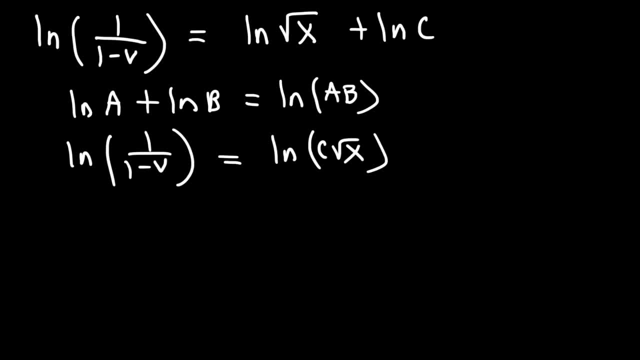 And on the left side it's just going to stay the same for now. So because we have a natural log expression on both sides of the equation and nothing else, we could set the integral inside of the natural log expression equal to each other. 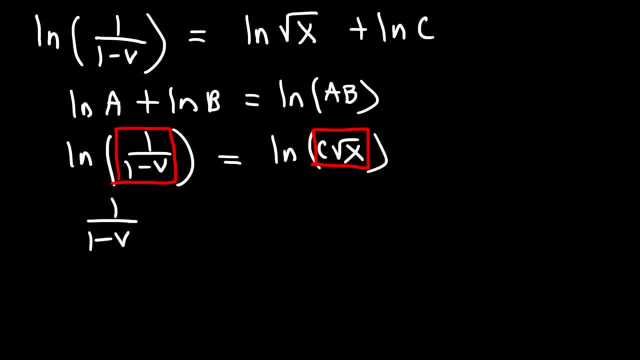 So therefore we could say that 1 over 1 minus v is equal to c times the square root of x. Now recall that we said y is equal to vx, So v is y over x. At this point, replace v with y over x. 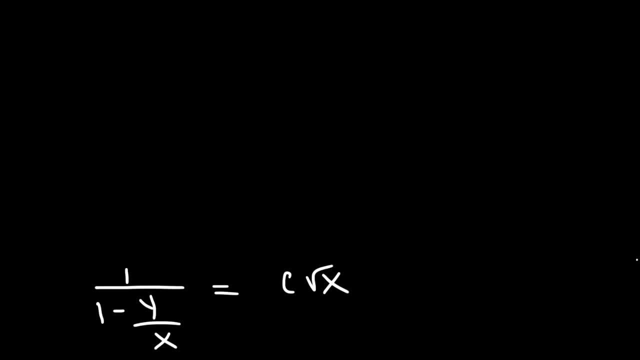 Because the original equation only had y and x. v was just a means to help us integrate the differential equation. Now, to simplify this complex fraction, I'm going to multiply the top and the bottom by x. So on the left I have x divided by. let's see: 1 times x is x. 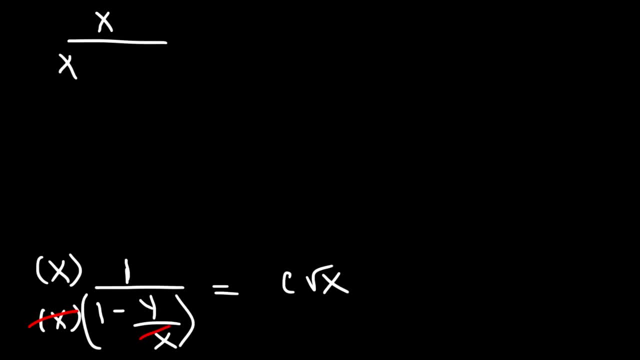 And then x times y over x, these will cancel, leaving behind negative y, And it's c. It's equal to c times the square root of x. Next, I'm going to multiply both sides by x minus y, And so these will cancel. 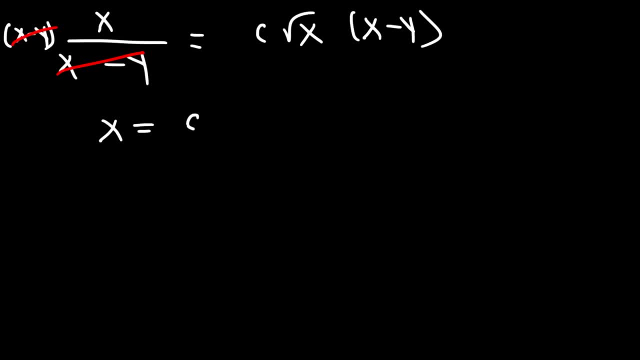 And now I'm left with x times c, square root: x, x minus y. Now, at this point, what you want to do is square both sides, So you have x squared on the left. Next you're going to have c squared. 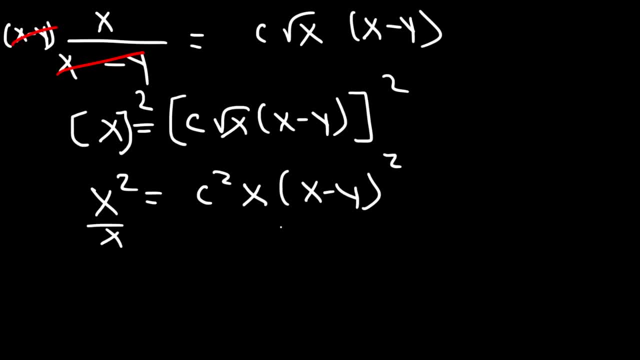 The square root of x squared is just x, And then x minus y squared. Now let's divide both sides by x, So these will cancel. On the left side, x squared over x is just x. Now c squared and c. they're both constants. 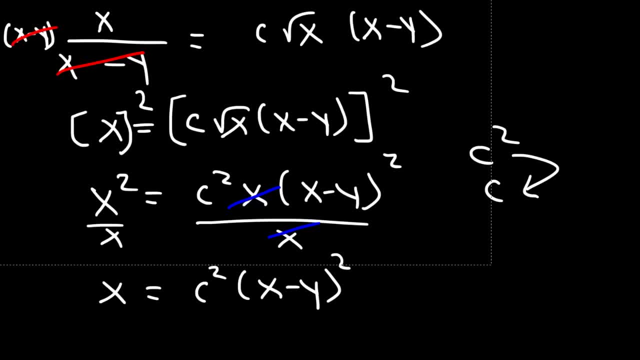 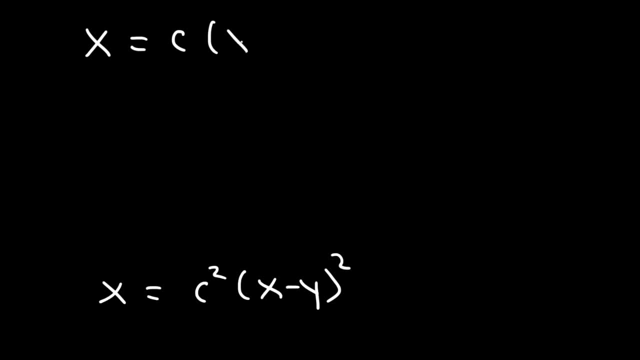 The derivative of c squared and the derivative of c is still 0.. So instead of writing c squared, you can it as y. choose us simply leave it as C, Just some generic constant. So right now we have: X is equal to C times. 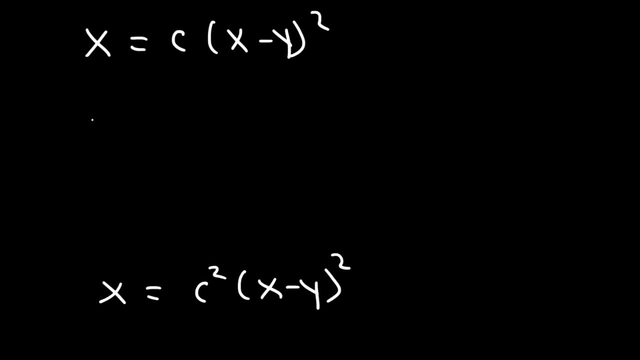 X minus Y squared. The final answer for this problem is as follows: The absolute value of X is equal to C times X minus Y squared. So this is the final answer. So that's the solution to the homogeneous differential equation. Now let's work on another example. 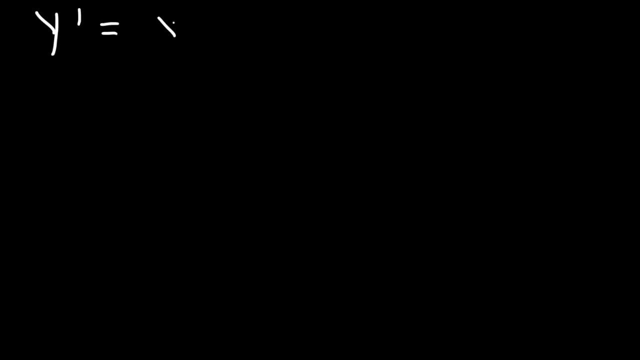 So let's say, if we have this problem, Y prime is equal to XY divided by X squared minus Y squared. So go ahead and solve this homogeneous differential equation. And the reason why it's homogeneous is because every term has the same degree. This term is degree 2, and 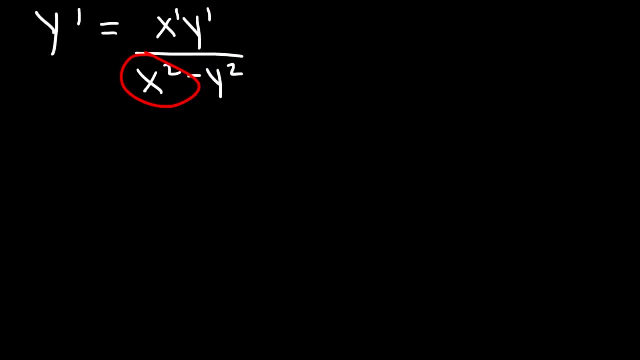 that's degree 2.. And then 1 plus 1 is 2.. So the first thing we're going to do is replace Y prime with DY divided by DX, And then we're going to put this in the appropriate form. So I'm going 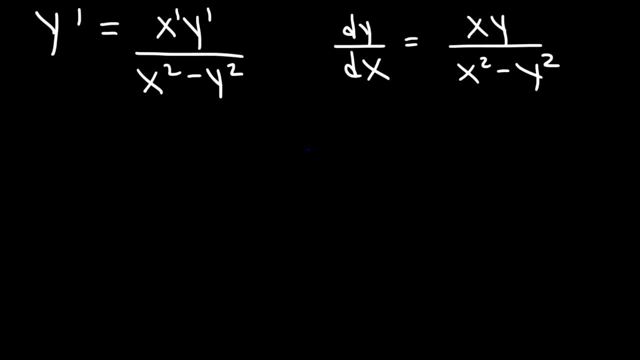 to FOIL, actually cross, multiply everything. So I have XY times DX and then that's equal to DY, DY times X squared minus Y squared. And so now that it's in this form, I'm going to replace Y with V times X, And just like: 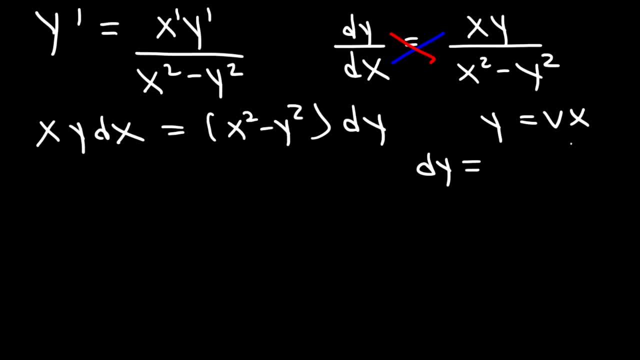 before. we know that DY is the derivative of VX. using the product rule, The derivative of V is DV, so we're going to have X- DV And the derivative of X is DX, so V times DX. So everywhere we see a Y, we're going to replace it with V times X And we're going to replace 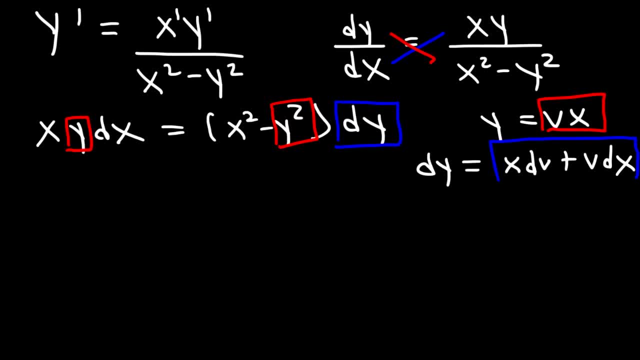 DY with X DV plus V DX, So this is going to be X times VX DX and that's equal to X squared. Now, if Y is V times X, Y squared is going to be V squared- X squared, So that's going to be V squared- X squared. 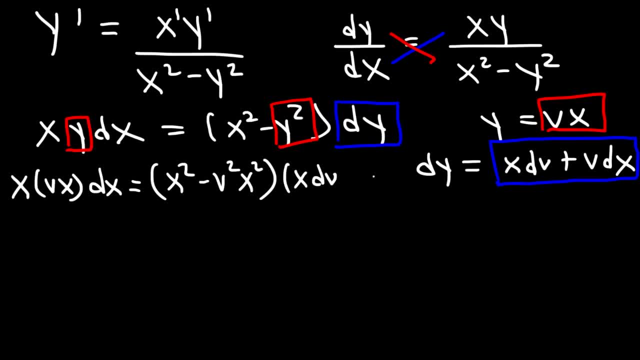 And then DY, which is X DV plus V DX. So on the left side, X times X, that's X squared. So we have V, X squared DX. Now on the right side I'm going to factor out X squared from those two terms. So I'm left with 1 minus. 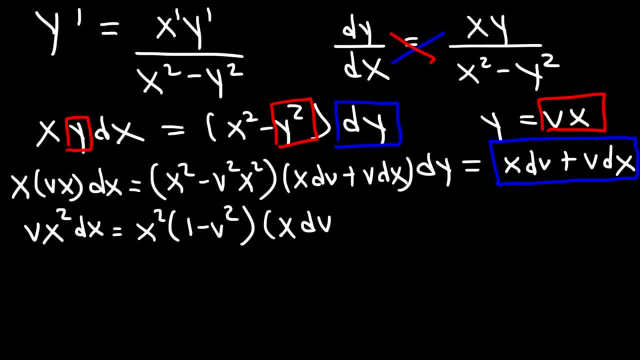 V squared, and I still have everything else: X DV plus V DX, X DV plus V DX. And let me just get rid of this. This is a different expression, Not a part of this one, So I just want to move that away so that there's no confusion. Now I can divide. 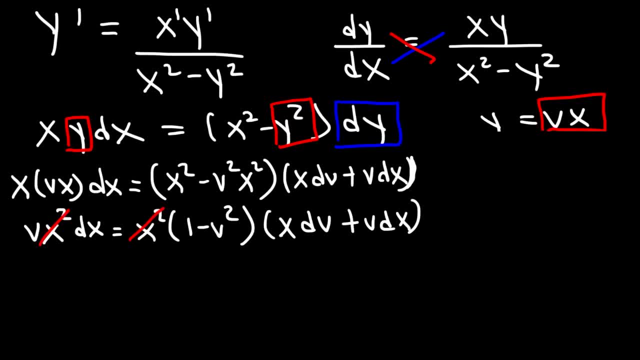 both sides by X squared, getting rid of this term. So on the left I just have V DX. On the right side we need to FOIL. So first we have 1 times X DV, So that's going to be X DV. 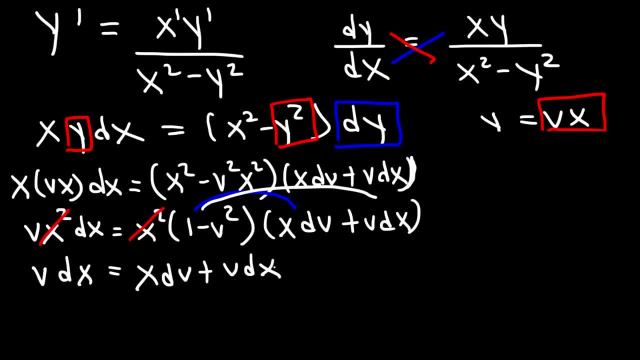 and 1 times Vdx, so Vdx, and then it's negative V squared times xdv. so negative xv squared dv, and then negative V squared times Vdx. so that's going to be negative V to the third power, dx. 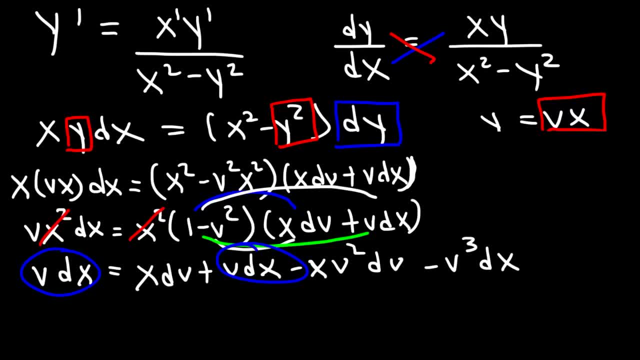 So notice that these two terms are identical. So, subtracting both sides by Vdx, they can be cancelled. Now what I'm going to do is take this term, move it to this side. So on the left side I have positive V to the third dx. 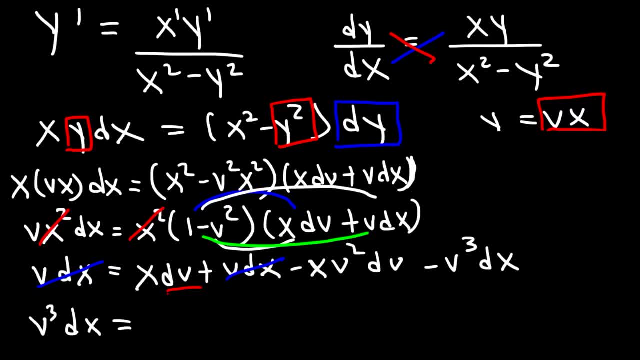 On the right side I can factor out an xdv. So if I take out x first, I'm going to be left over with 1 minus V squared and I have to take out dv. but I'm going to write it at the end. 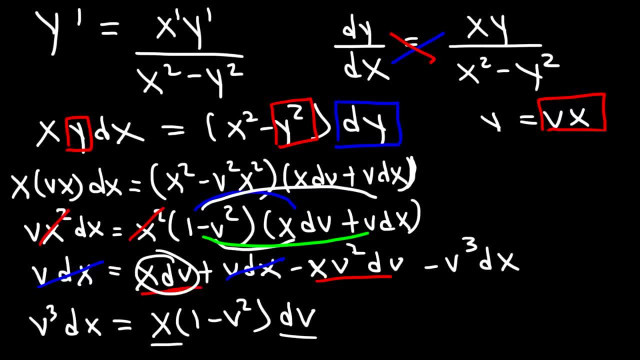 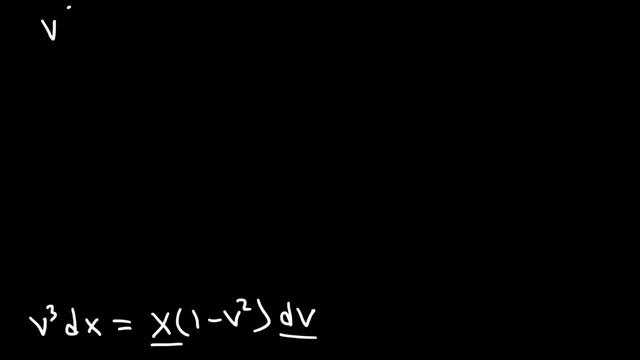 So I took out xdv first From this term, which leaves a 1, and taken out from this term, it leaves behind negative V squared. Now I'm going to rewrite what I have at the top. So that's V to the third dx. 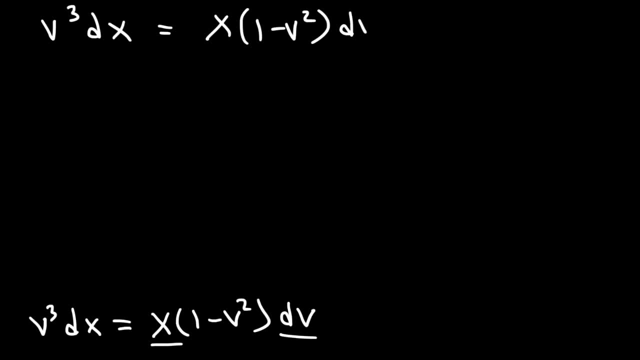 It's equal to x times 1 minus V squared dv. So at this point we need to separate the variables, So we need to put x on one side and v on the other. So I'm going to, So I'm going to divide both sides by V to the third, and at the same time I'm going 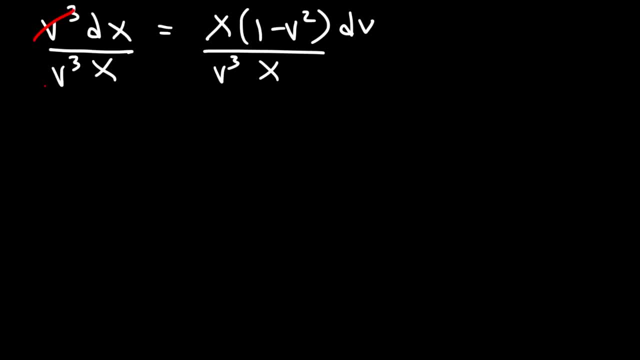 to divide it by x. So on the left side V to the third will cancel and on the right side x will cancel. So on the left I have 1 over x dx and on the right that's equal to 1 minus V squared. 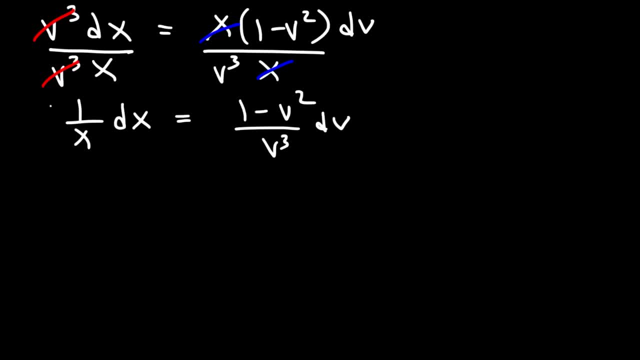 divided by V to the third dv. So at this point we can take the integral of both sides. Now, on the right, we need to separate the variables. So we're going to separate it into two integrals: 1 divided by V to the third. 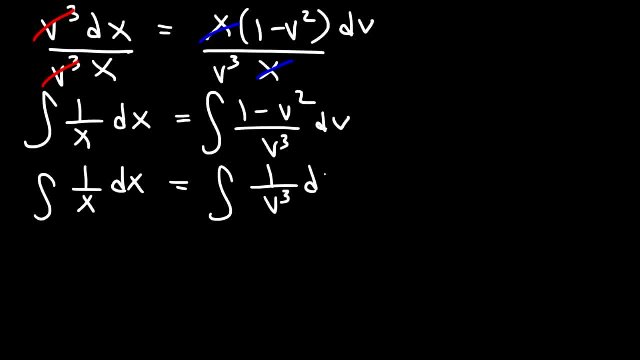 So we have the integral of 1 over V to the third dv and then minus V squared over V to the third. So that's going to be the integral of 1 over V dv. So let's focus on this integral. first We need to rewrite it. 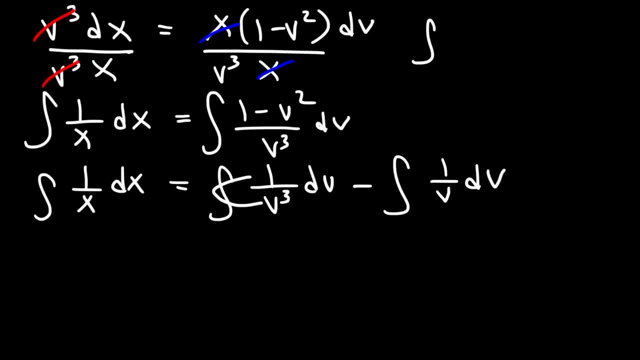 We need to move V to the third, from the bottom to the top. So this is the integral of V to the negative 3.. And using the power rule, we're going to add 1. To negative 3.. So negative 3 plus 1 is negative 2, and then divide by that result. 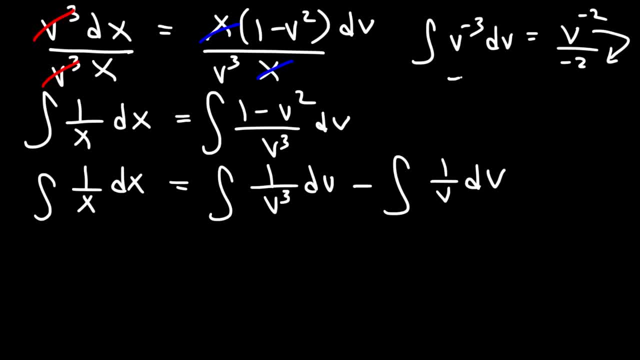 Now I'm going to bring V back to the bottom. So it's negative 1 over 2 V squared. Now the antiderivative of 1 over x is ln x, And this we said, it's negative 1 over 2 V squared. 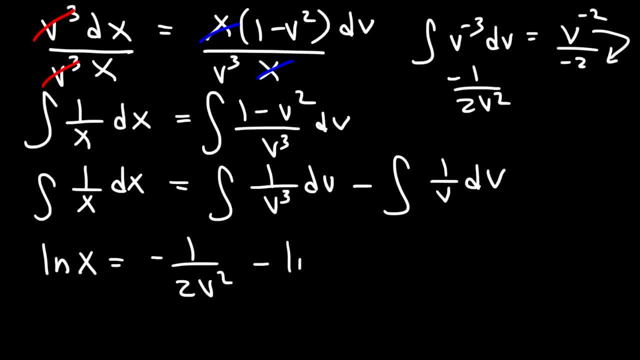 And the antiderivative of 1 over V is going to be the natural log of V and then plus C. So right now we need an absolute value in front of x and V. Now let me delete a few things to make more room. 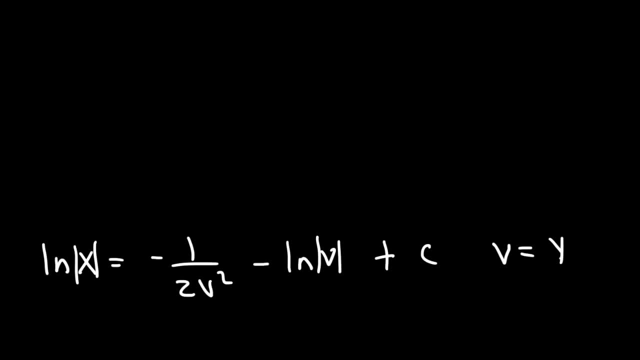 So at this point we're going to replace V with y over x. Keep in mind: y is V times x, So V is y over x. So we have the natural log of x and that's equal to negative 1 over 2 times y over x. 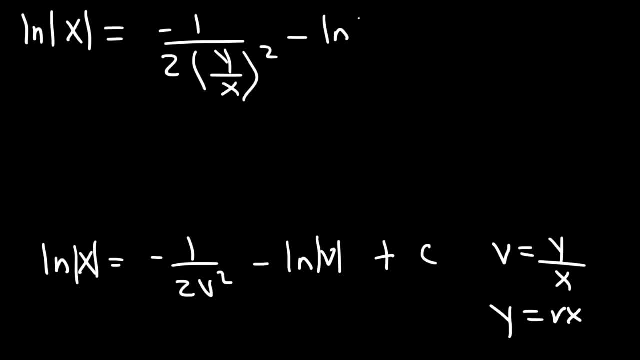 And then minus ln V, and that's ln y over x plus C. So this is going to be y squared divided by x squared. Now recall that we said ln A plus ln B is ln A times B. So ln A Minus ln B is going to be ln A divided by B. 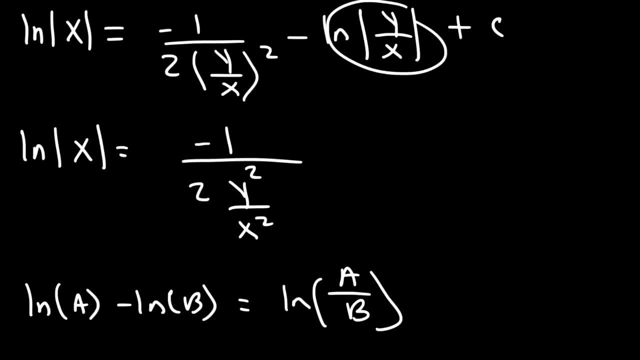 So therefore, we can replace ln y over x with ln y minus ln x, which is what we're going to do in the next step. So this is going to be minus and then ln y, minus ln x and then plus C. 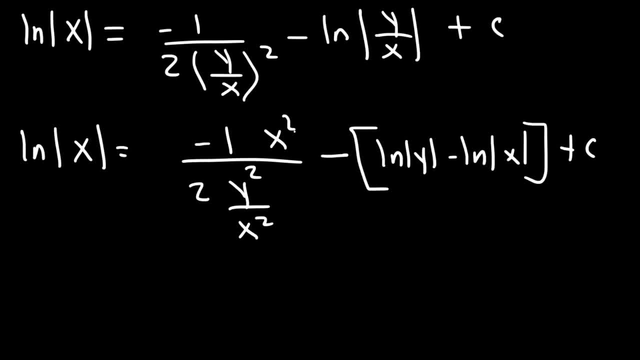 Now for this fraction. let's multiply the top and the bottom by x squared. So we can. So we can Simplify this complex fraction. So right now we have ln x, that's equal to negative x squared, divided by 2y squared. 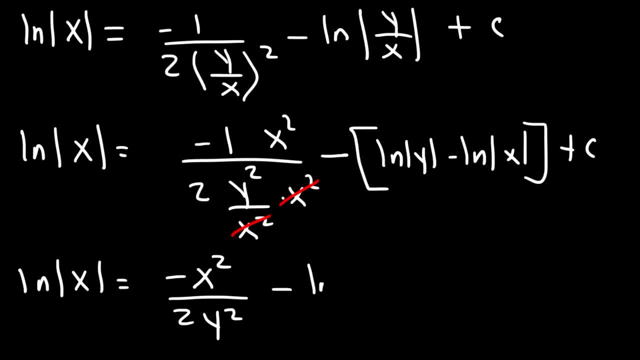 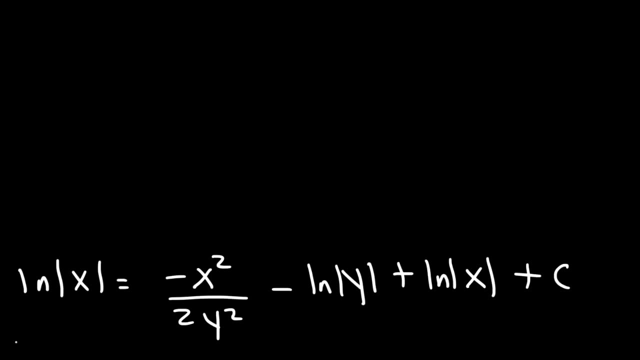 And now we need to distribute the negative sign. So it's a negative ln y plus ln x plus the constant C. At this point we can subtract both sides by ln x, If we do. If we do, these terms will cancel. 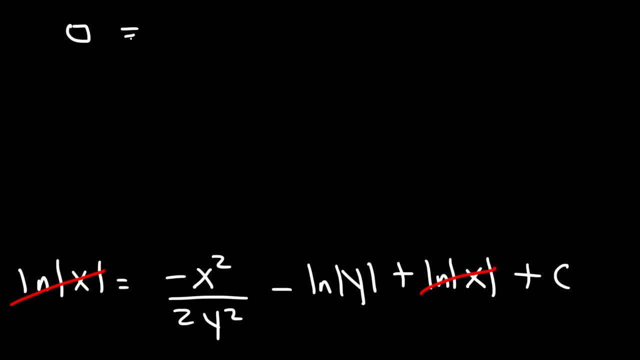 And so right now we have: 0 is equal to negative, x squared over 2y squared minus ln y plus C. Now I'm going to take ln y, move it to this side, So it's going to be positive on the left side. 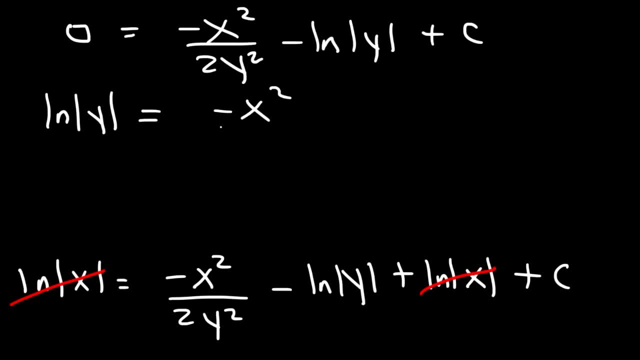 So ln y is equal to negative x squared over 2y squared plus C. Now, what I'm going to do is put everything- I'm going to put everything- on the exponent of E. So on the left side it's going to be E to the ln y. 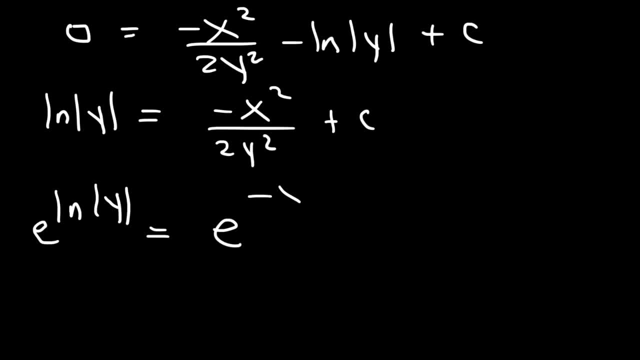 On the right side it's E to negative, x squared over 2y squared plus C. Now E raised to the ln y, the E's will cancel And for the most part we're just going to get y. Now on the right side we have two terms that are added on the exponent of E. 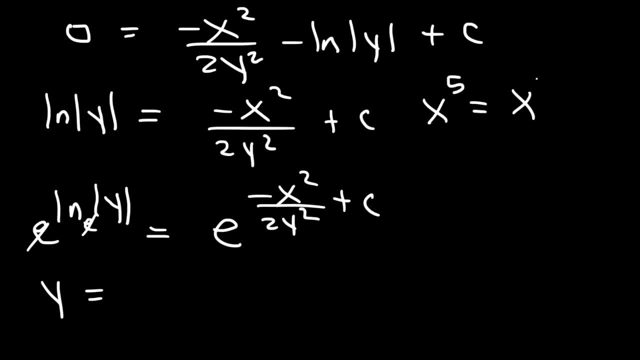 Now, for instance, let's say, if we have x to the 5. 5 is 2 plus 3.. And we know that x to the 5 is x squared times x cubed. So what I can do is take this and split it into two parts, which is what I'm going to do with E. 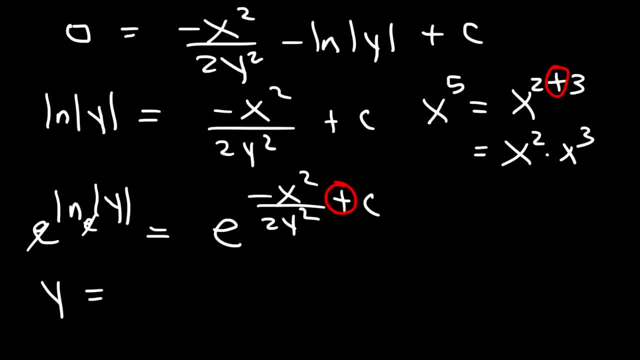 Since there's a plus sign between the C and the negative x squared over 2y squared, So I can write it as E to the negative x squared divided by 2y squared times. There's a multiplication here: E to the C. 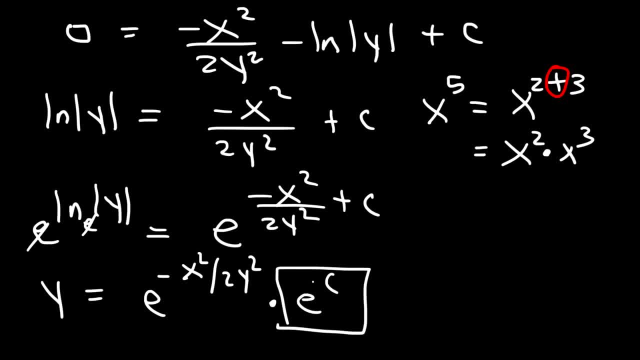 Now E to the C, a number raised to a number, that's a constant. So I could just replace that whole thing with C And I'm going to move that to the front. So the final answer for this problem is: y is equal to C. 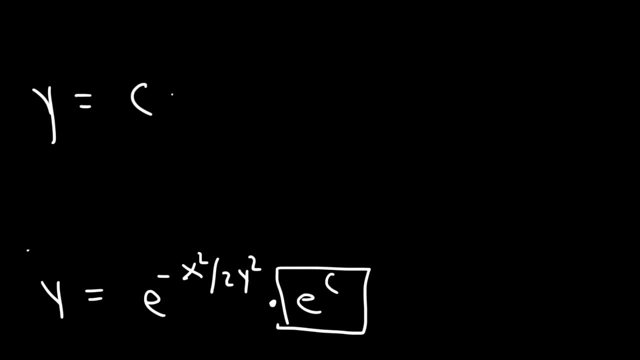 Let me rewrite that here I need more space. And then times E raised to the negative, x squared over 2y squared. So that's the final solution for this Homogeneous differential equation. That's the answer. Let's work on another problem. 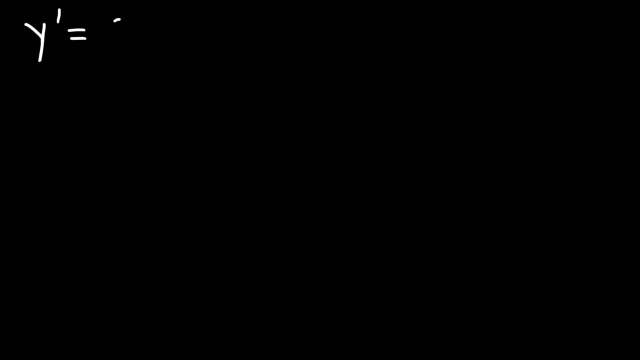 So let's say that y prime is 2x, E raised to the negative, y over x plus y divided by x. And let's say we're given a point 1 comma 0. So we got to find the value for C, So go ahead and solve this differential. 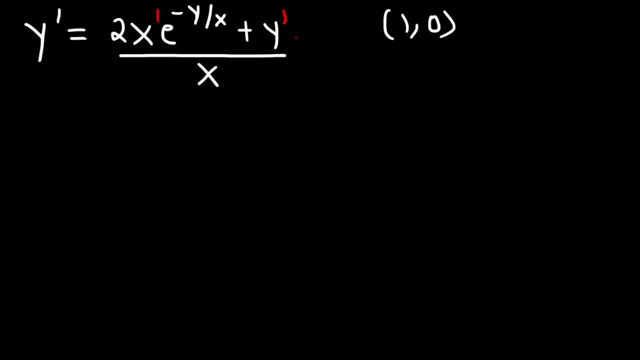 Now, every term is to the first degree, And this exponential part of this term it doesn't matter. so to speak, It's not counted. So this is a homogeneous differential equation. We can use the same process to integrate it. So what we're going to do first is replace y prime with dy over dx. 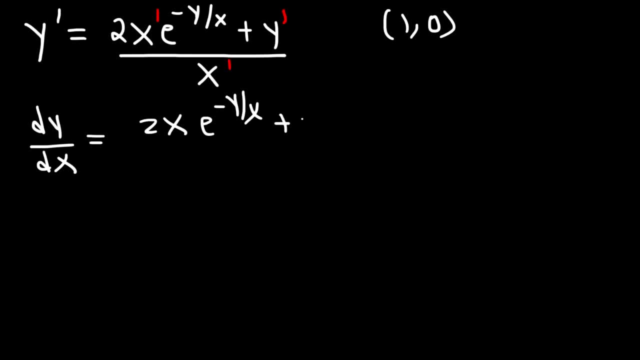 And let's cross multiply. So we're going to have x times dy on the left side And then on the right side it's going to be 2x E raised to the negative y over x plus y, And then times dx. 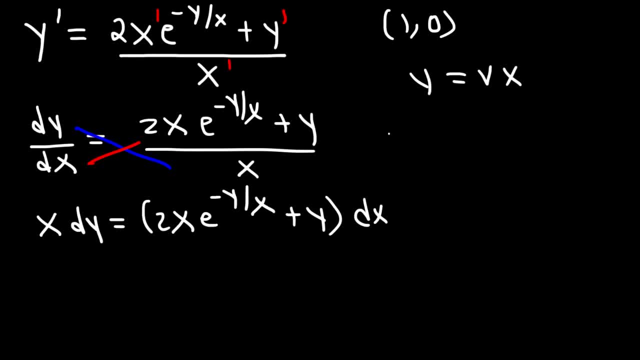 So, as always, we're going to replace y with v times x. So dy is going to be xdv plus vdx. Now let's replace dy with this expression, And then everywhere we see a y variable, here and here we're going to replace it with v times x. 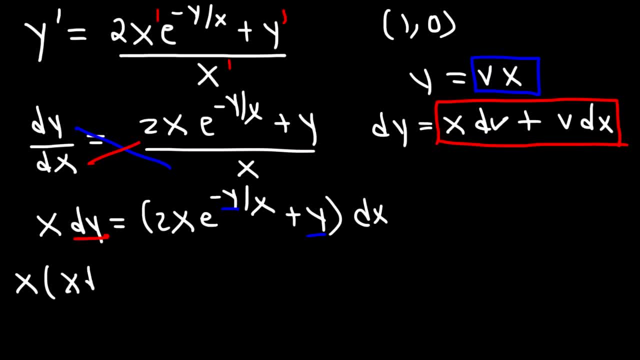 So this is going to be x times xdv plus vdx And that's equal to 2x. So we're going to have 2x E raised to the negative vx divided by x, and plus another vx, dx. So on the left side, I'm just going to rewrite what I have. 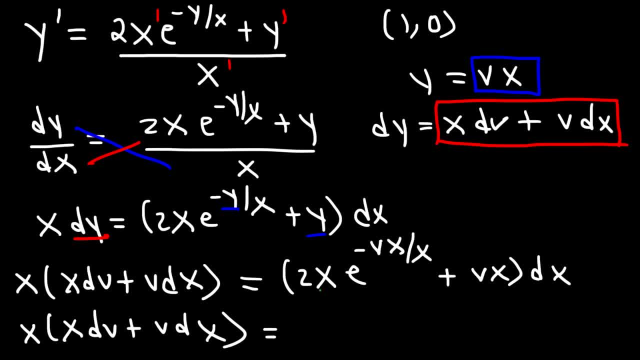 On the right side notice that I can factor out an x And at the same time this x variable will cancel. So I'm going to have x times 2E to the negative v plus v times dx, So at this point I could divide both sides by x. 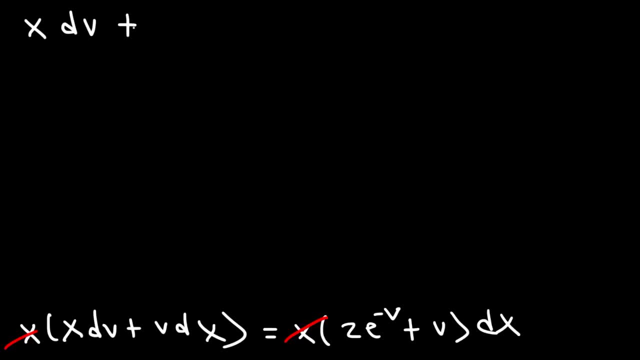 So on the left side, I'm left with xdv plus vdx And that's equal to 2E to the negative v. Well, I'm going to distribute dx to these two terms. So this is going to be 2E to the negative v dx. 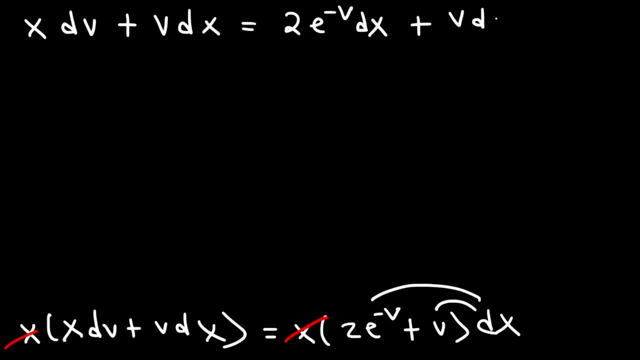 And then that's going to be 2E to the negative v dx plus V DX. so notice that these two terms are the same. so if I subtract both sides by V DX, they will cancel, and so I'm left with X DV and that's equal to 2 e. 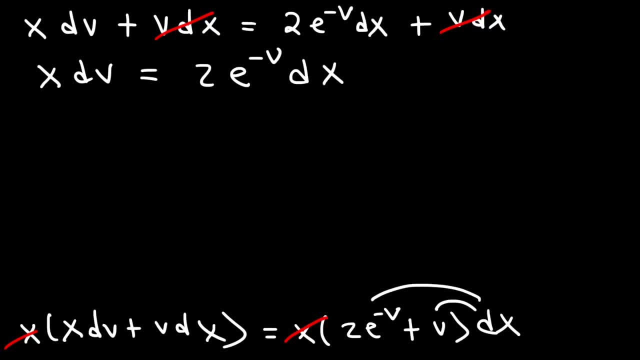 negative V, DX. at this point we need to separate the variables. so let's divide both sides by X and at the same time by 2 e to the negative V, so we could cancel 2 e to the negative V on the right side, and on the left we can cancel X. so on the 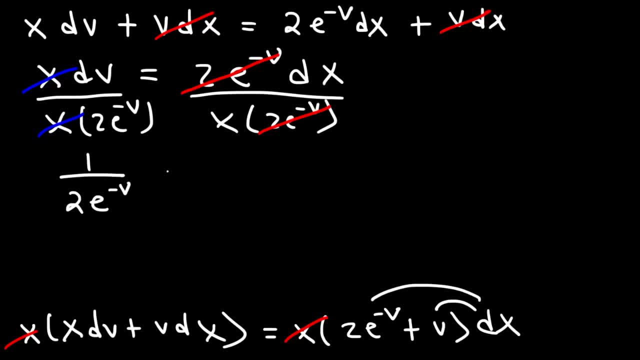 left side I have 1 divided by 2 e negative, V, DV, and on the right side I have 1 over X, DX. so now what I need to do is move the e to the top to make the negative exponent positive. So I have e. let me change the color. 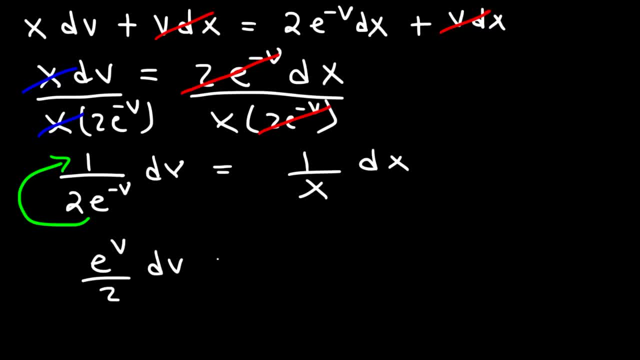 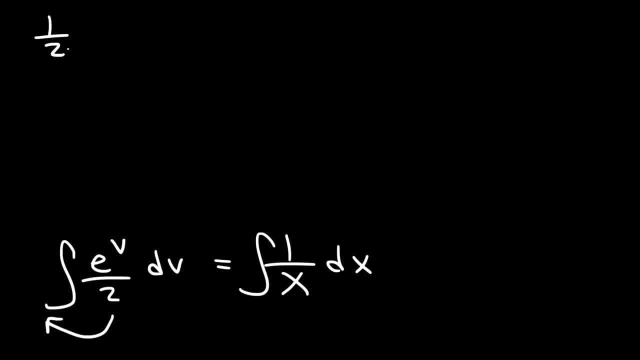 so e to the positive v divided by 2 dv, and that's equal to 1 over x, dx. So now I could take the integral of both sides. So I'm going to move this constant to the front. So I have 1 half the integral of e to the v. 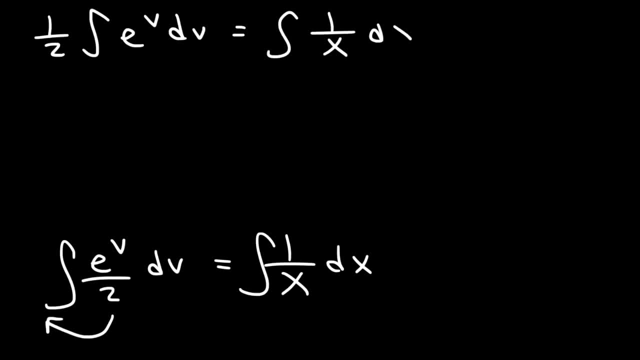 dv, and that's equal to the integral of 1 over x dx. The antiderivative of e to the v is just e to the v, but times 1, half in this case, And the antiderivative of 1 over x is ln x plus c. 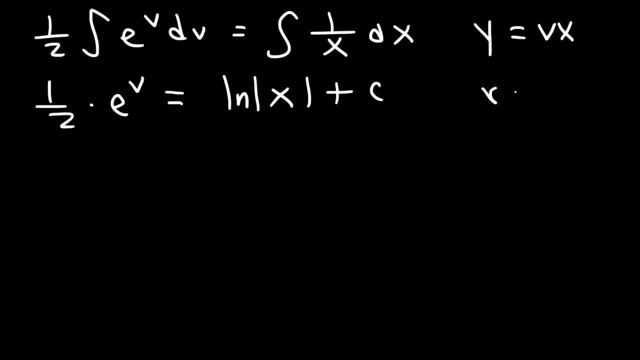 So now we said that y is equal to vx, So v is y divided by x. So this is going to be e raised to the y-th, And that's equal to ln x plus c. So at this point I'm going to multiply both sides by 2.. 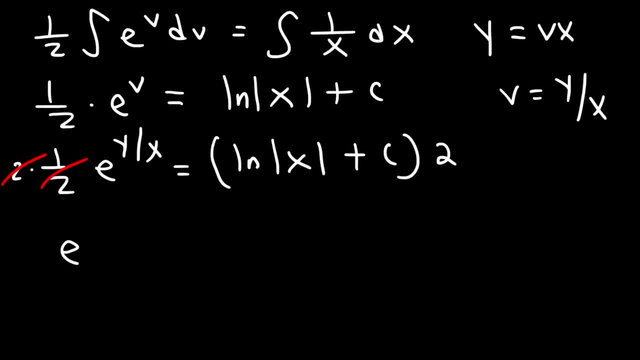 2 times 1 half is 1.. So on the left side I just have e raised to the y over x, And on the right side I'm going to have 2 ln x plus 2c. Now for 2 ln x, I'm going to move the 2 to the x-th. 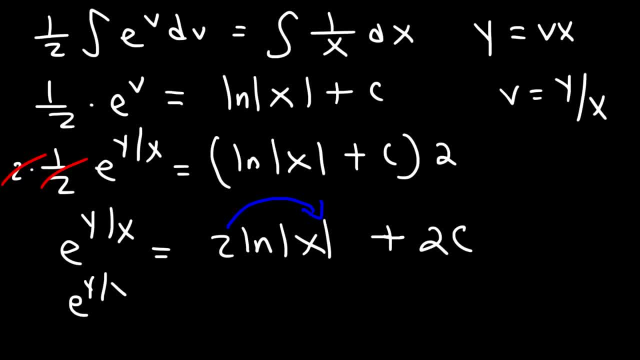 So this is going to be e to the y over x, and that's equal to ln, x squared. x squared is always positive, so I no longer need the absolute value symbol And 2c is a constant, so I can replace that with c. 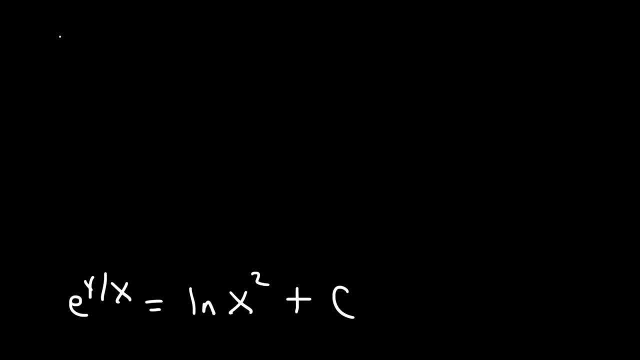 And so this is the general equation, or the general solution of the differential equation. So e raised to the y over x is equal to ln x squared plus c. Now the only thing that's left for me to do is to calculate the value of c. 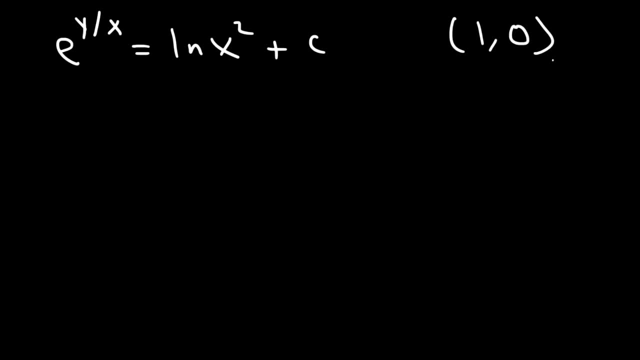 Now recall that we have the initial value, or the initial point, 1 comma 0. Which means that when x is 1, y is 0. So let's plug in x and y. This is going to be e to the 0 divided by 1, and that's equal to ln 1 squared plus c. 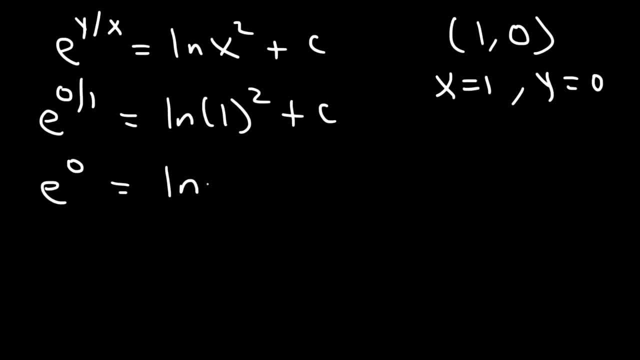 0 divided by 1 is 0, and 1 squared is 1.. e to the 0 is 1.. ln: 1 is 0. So we can see that c is equal to 1.. So now that we have the value of c, we can write the final answer. 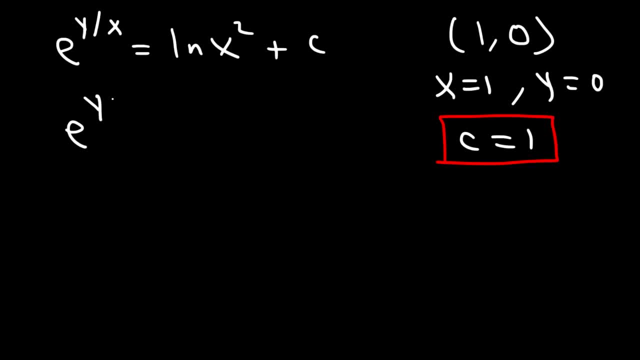 So we can say that e raised to the y, divided by x, is equal to ln x squared plus 1.. Or we can write that like this: It's equal to 1 plus ln x squared, And so this is the final answer. That's all. 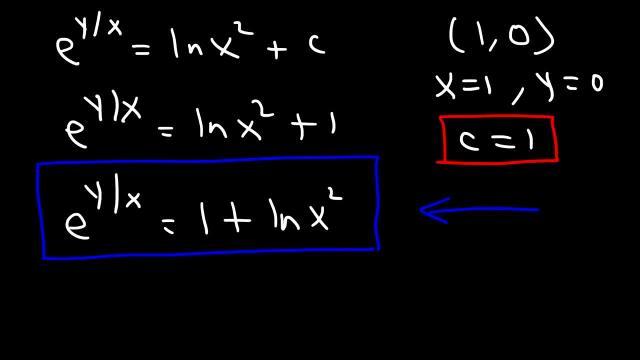 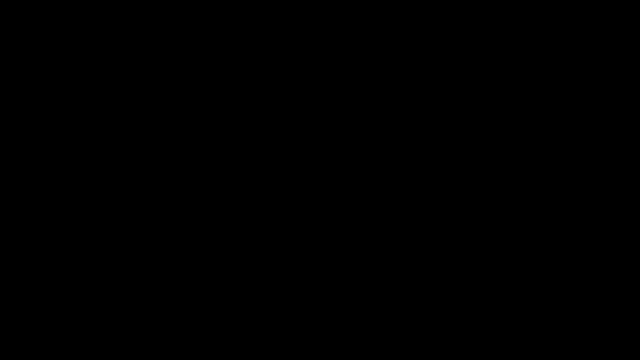 That's all we need to do in this problem. So that's it for this video. Now you know how to solve a homogeneous differential equation. Thank you.